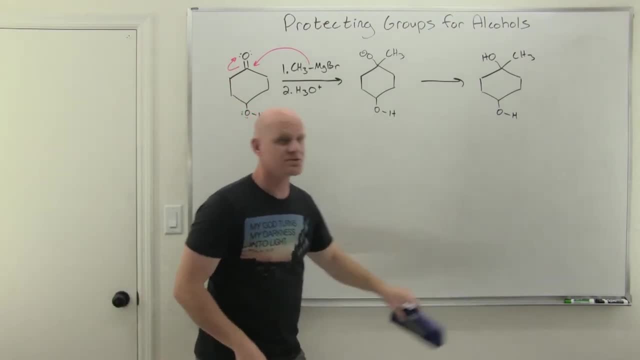 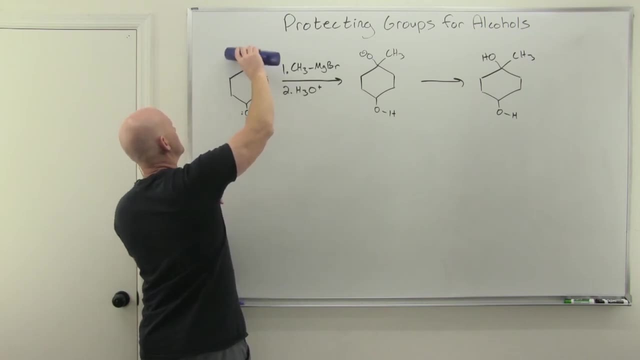 which is what we wanted to do, but it's also a strong base, And so the truth is, it is never going to get a chance, in this case, to react as a nucleophile, because the acid-base reaction is typically faster. 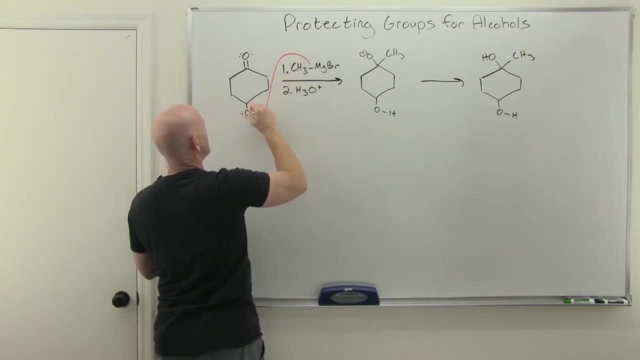 And so, as a result, it's going to come down here and deprotonate that alcohol. So, and as a result, you're actually just going to get ketone's. still going to be a ketone, You're going to form this alkyl oxide. 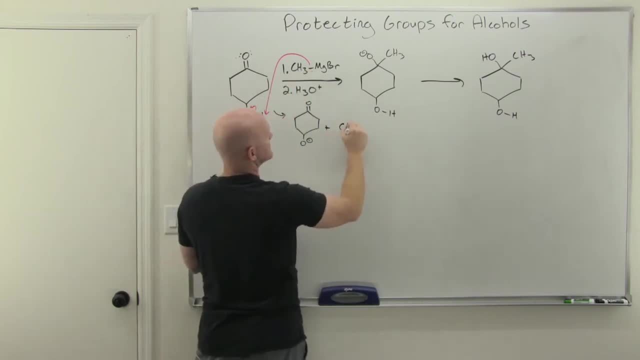 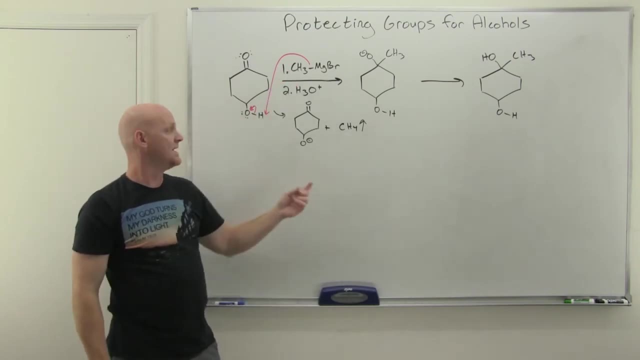 When the CH3 here bonds to another H, that becomes CH4, which in this case is methane, which is a gas and just bubbles out of the solution. And so your Grignard's just been consumed, turning into methane, and all you've done. 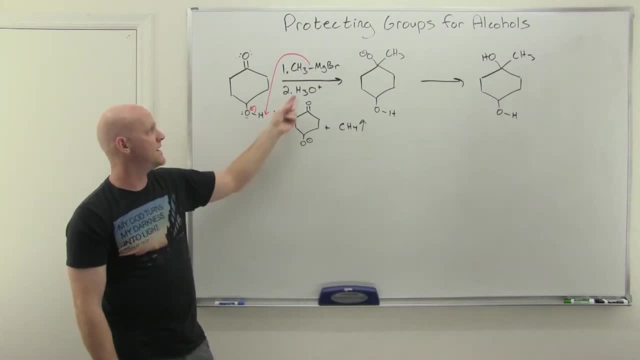 is deprotonate your alcohol effectively, turning it into alkoxide. When you add the H3O+, it'll just turn it right back and you'll be back to where you started with and you've done nothing. So in this case, we need to first protect this alcohol here in order for this reaction. 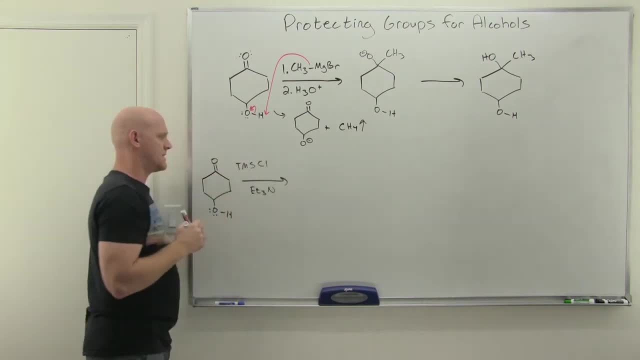 to work, So let's take a look at what this looks like here. All right, so the reagent we're going to use here is called trimethylsilyl chloride. There's our abbreviation, and we're going to need a base in there, and oftentimes we'll 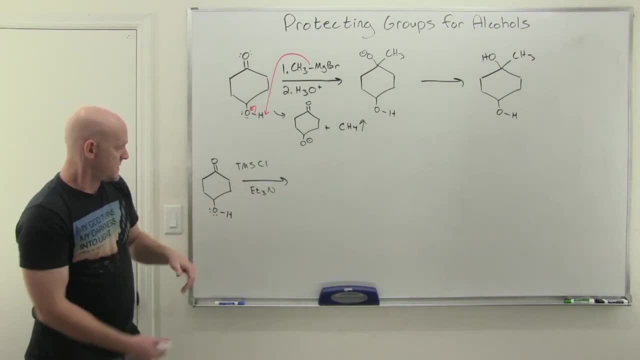 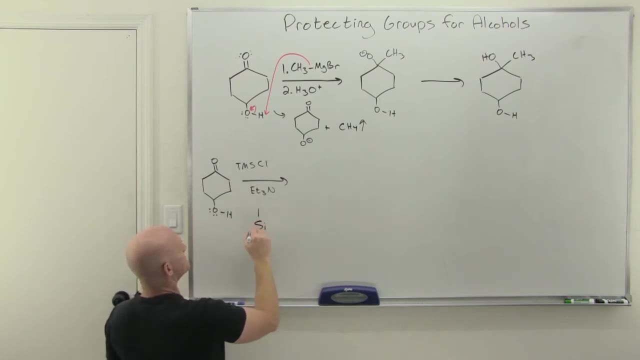 use like triethylamine or maybe pyridine, as we'll see. So, and in this case, the way this works, if we draw this out. so this trimethylsilyl ether, the silyl refers to silicon trimethyl. that's what we got going on here, and then 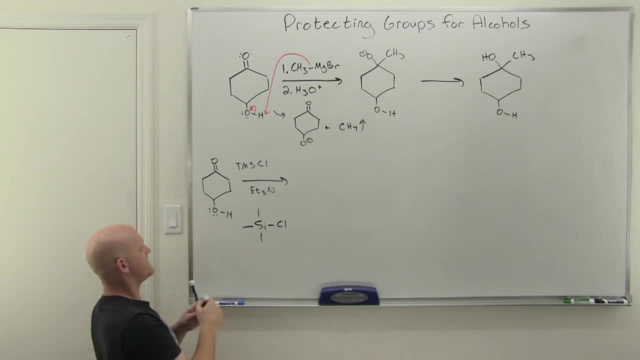 chloride here And the chloride here is just a leaving group, And what we're going to have happen here is we are going to attack the silicon and have the chlorine And I'm going to make this look very SN2, and you might, for a second, be like Chad. 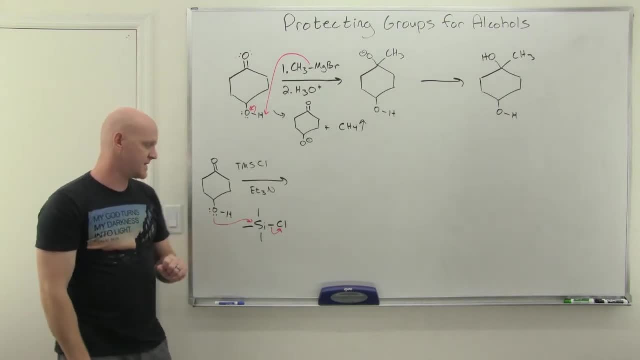 you can't attack a tertiary with SN2.. You can't attack a tertiary carbon with SN2.. But silicon is bigger, which means these three methyl groups are going to be farther apart and a nucleophile actually can squeeze in to attack the larger silicon. 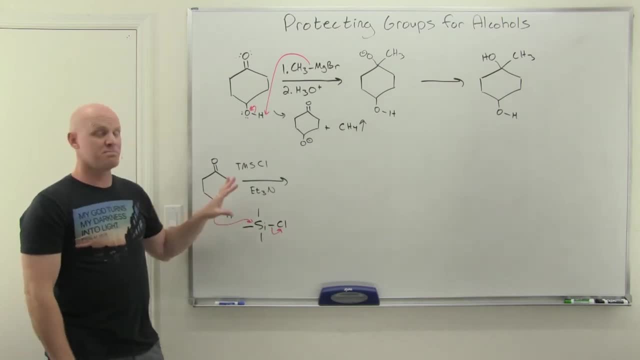 If this were a carbon- you're right- could attack it. So also the truth is this probably actually isn't SN2.. So good evidence that shows that this might actually go through what's called a pentavalent intermediate. So pentavalent means silicon would have five bonds. 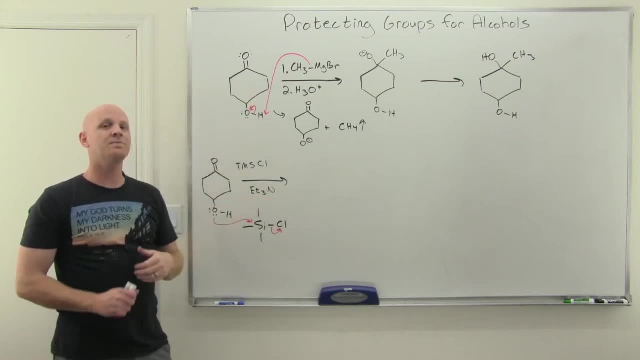 For a spell. Silicon's in the third row of the periodic table, and it's allowed to go over the octet rule, And so the truth is the oxygen probably bonds first and then, in a separate step, the chlorine will leave. 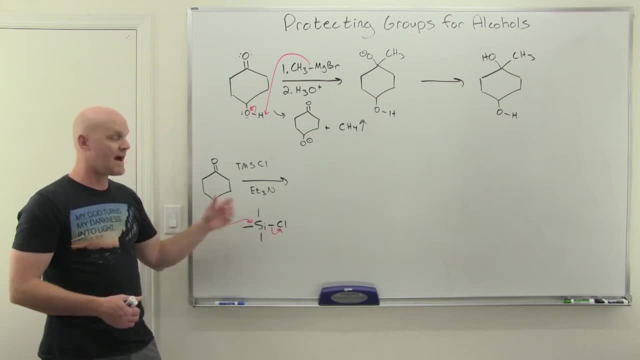 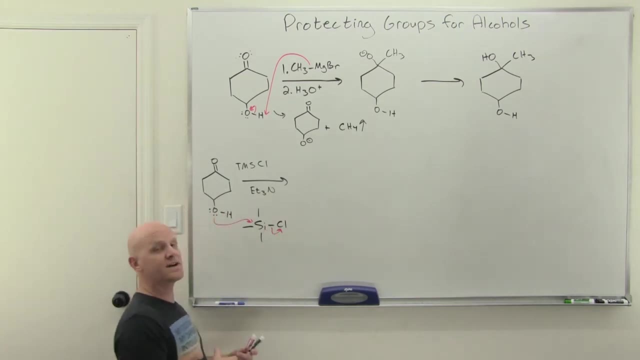 So well, before the chlorine actually leaves, we'd end up with this silicon having five bonds for just a minute. But we're not going to show that here, So we're just going to kind of show the SN2-like step and you'll see it kind of presented. 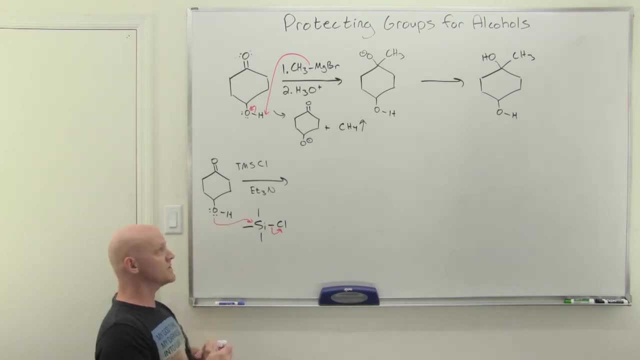 both ways, And the truth is it might even be more complicated than either of those. There might be competing mechanisms going on and things of this sort, But usually the mechanism is not The point of focus here. most of you aren't even going to see a mechanism presented for. 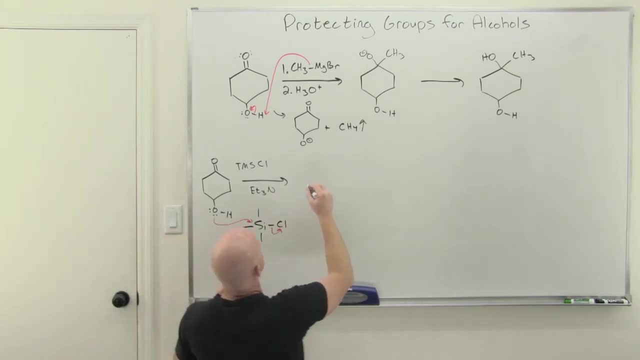 this reaction. So I just wanted to make sense for you. So in this case, this will take us now to our ketone. with this oxygen, now bonded to silicon, still has a hydrogen. So and that's where our lovely base here, the triethylamine, comes into play. 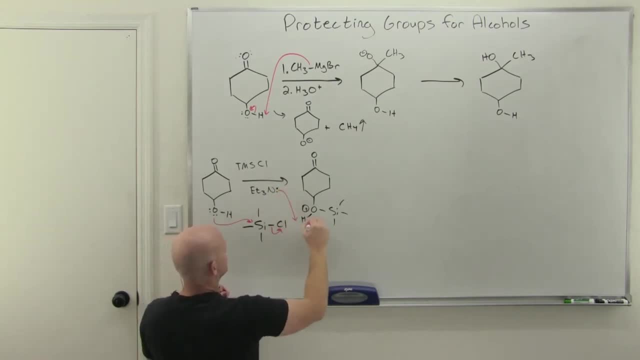 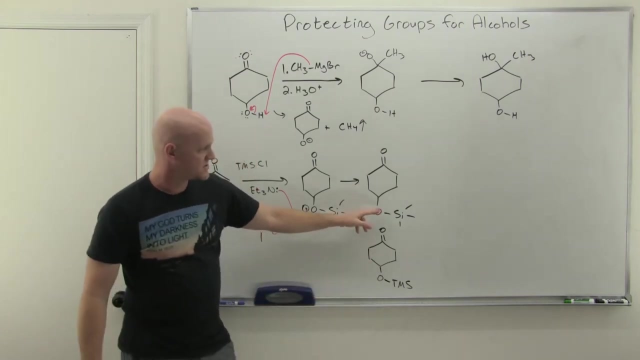 It's just there to deprotonate this hydrogen. So in this case you might see this abbreviated like so, or just simply written OTMS or something like this. So same kind of thing. I just want to make sure you've seen both what it looks like in actuality as well as. 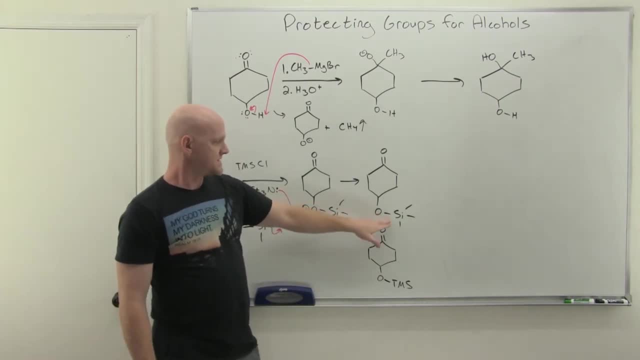 the abbreviations commonly used, so you can relate the two. So, but this is nice. It's actually a reversible reaction. We'll find out how we can remove this when we're done. But what's nice is temporarily there's no hydrogen bonded to our oxygen. 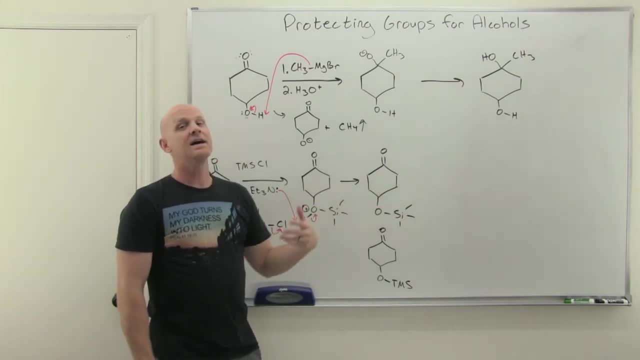 It's not an alcohol anymore. There's no acidic hydrogen down here whatsoever, And so if we had a Grignard now, it's not going to react as a base. The only option it actually has is to act as the nucleophile, like we want it to. 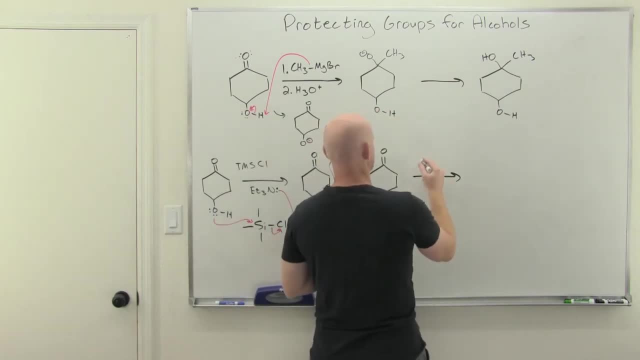 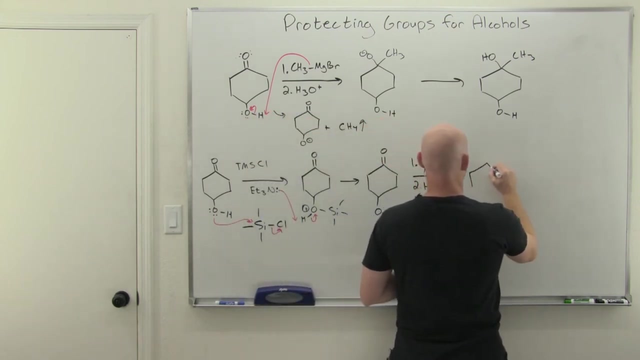 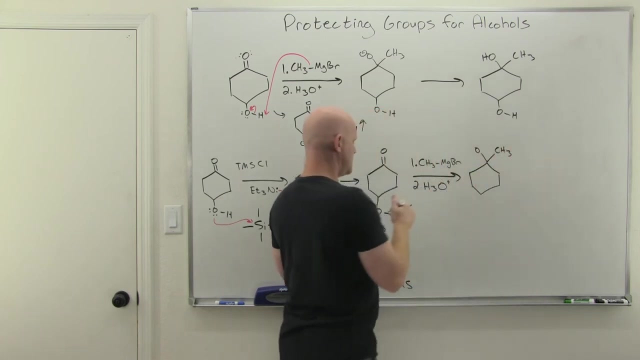 And so that's what we're going to do here. Cool, and I'm going to write that out, just like we did here. So we'll find We've attached our new methyl group here. It's just coming in attacking as a nucleophile, like we wanted it to. 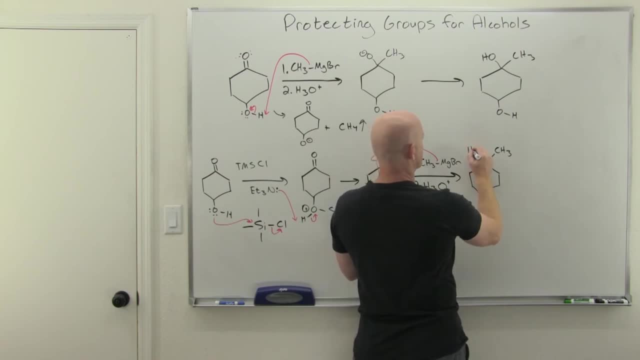 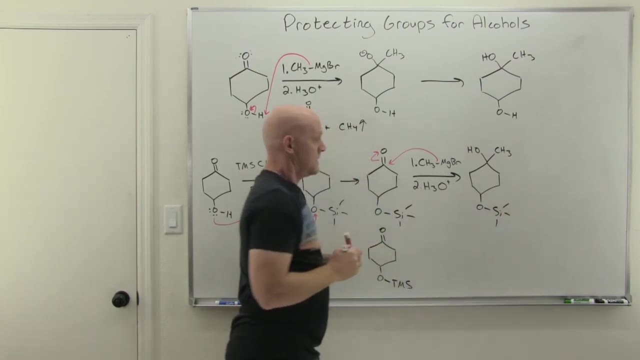 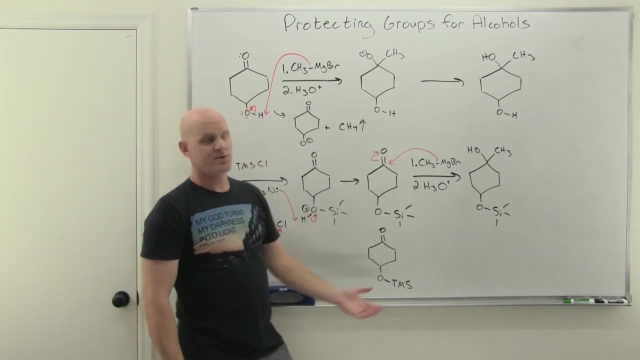 So forming the alkoxide, then the H3O plus is going to protonate. that Cool, But it turns out That might not be the only thing that happens If we make this H3O plus concentrated enough. So it turns out. H3O plus is one of the couple of ways you'll learn to deprotect this. 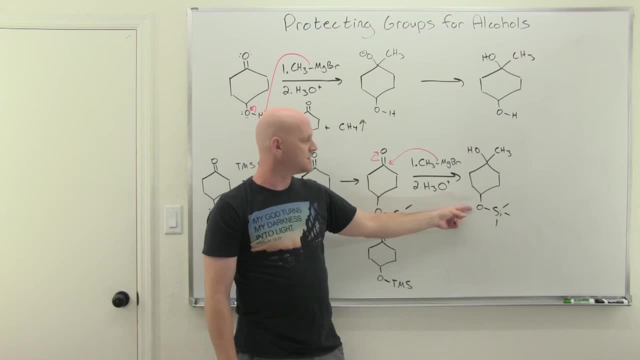 It'll actually hydrolyze this. You'd end up protonating this oxygen, putting an H back on there, So, and then you'd probably have water coming and attacking the other side and breaking the bond off And you'd be back to having an alcohol. 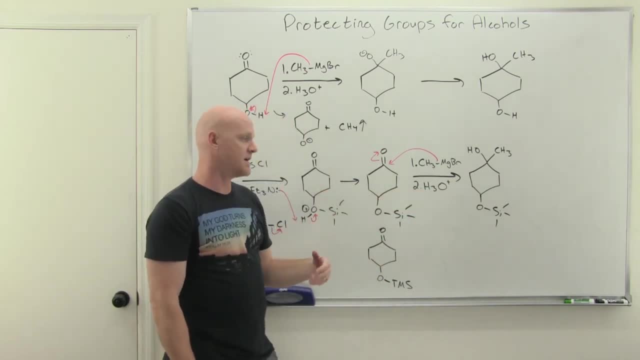 And so the truth is, if your H3O plus is concentrated enough, So this would already be back to an OH. So, however, if it's not concentrated enough, Well now you could make it more concentrated, I guess. So, but the other thing you might do, 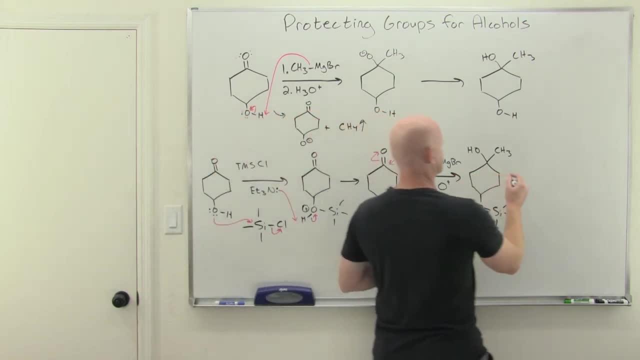 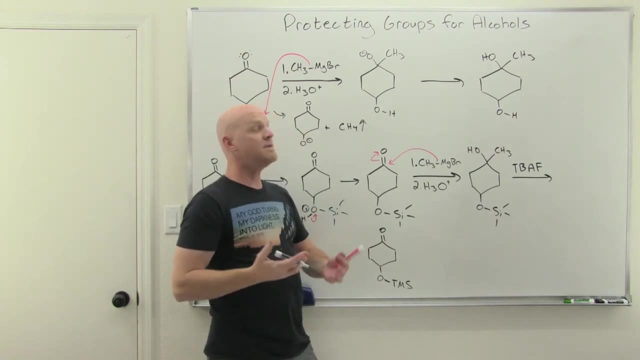 And it's probably the more common deprotecting agents, What's called TBAF, So abbreviated TBAF, Most commonly written as TBAF. You may never even see its structure formally drawn out, Or at least not very often. 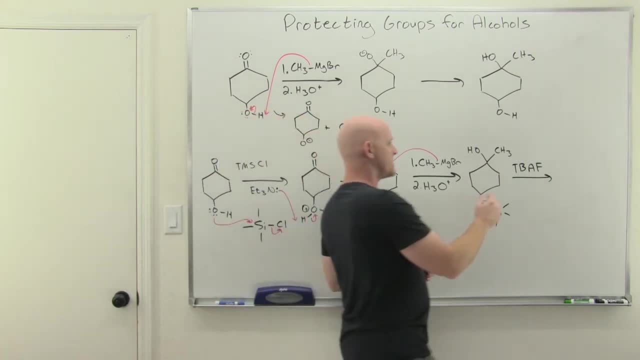 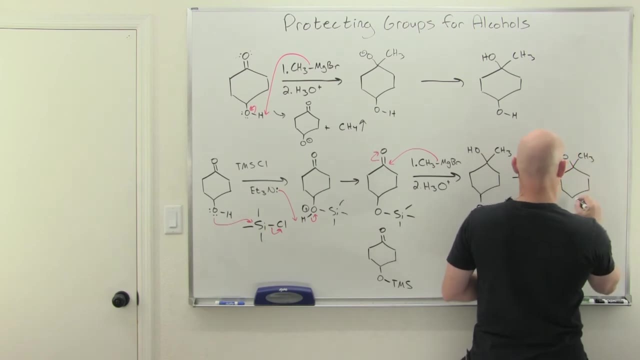 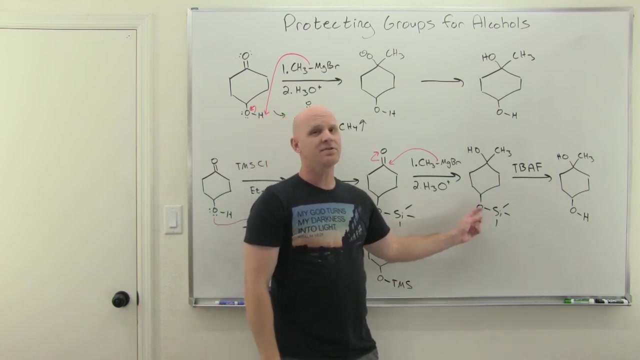 Except maybe in an explanation. So you're probably going to see that abbreviation more than anything else. So, but that TBAF is more commonly used here. Here, And gets us back To our alcohol. Now the truth is the trimethyl siloether is not the only kind of siloether you might use. a protecting group. 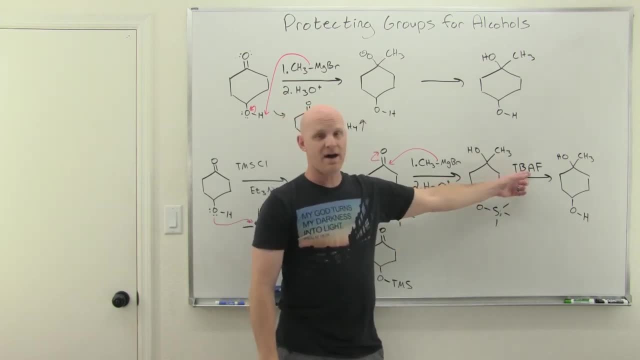 And the bulkier these groups get, The more you actually need TBAF. So H3O plus will work with trimethyl siloether- Some of the bulkier ones. it won't, And you have to use TBAF, And so that's why I want to take the time to use it here. 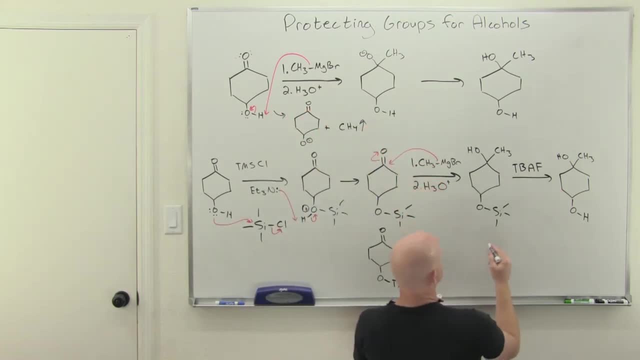 But TBAF stands for tributyl. I'm sorry, tert-butyl. Let's try that, Let's get that right, Let's draw that a little prettier, Okay, so there's tert-butyl-ammonium, tert-butyl-ammonium. 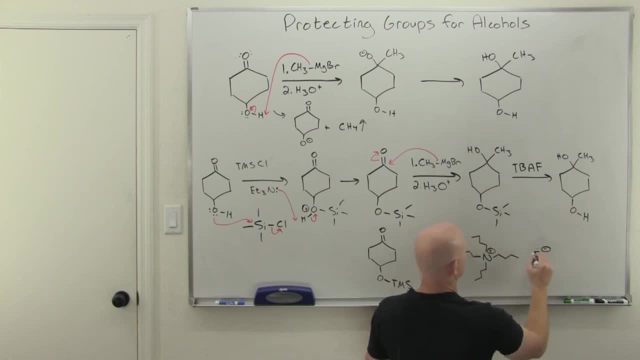 But the important part here is fluoride. Don't care about the tert-butyl-ammonium part. This is just a way of getting fluoride ion in the solution with something big, organic-y and making it soluble and a lot of organic solvents, But the fluoride is the key. 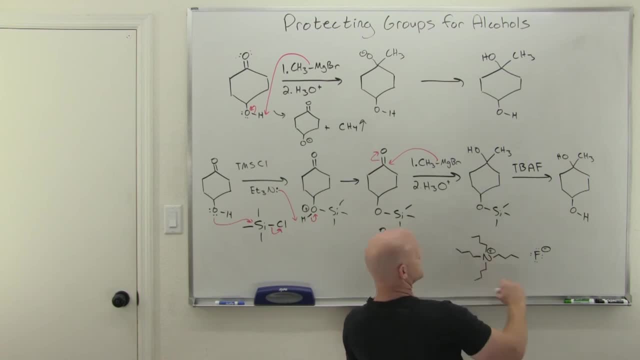 And the idea is that we're eventually going to- turns out, this is always going to be present- with a little bit of water, So, and that water is going to approach, Protonate this oxygen here, And then fluoride is going to come in and do backside attack.